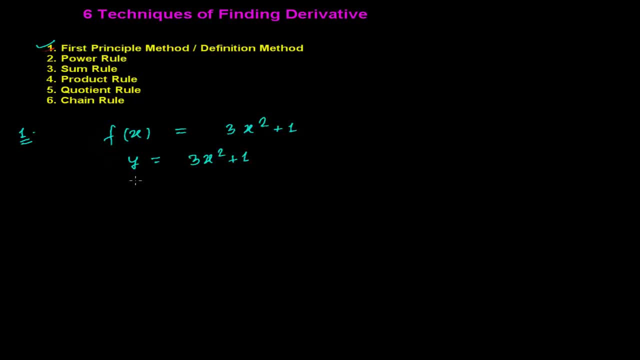 I'm just making a small change in y as well as in x, right, So y plus delta y And similarly in x. also a small change is going to be there: x plus delta x, whole square plus one. And then we used to shift this y to right side. then I can write: delta y equals to three x square plus two x delta, x plus delta y. 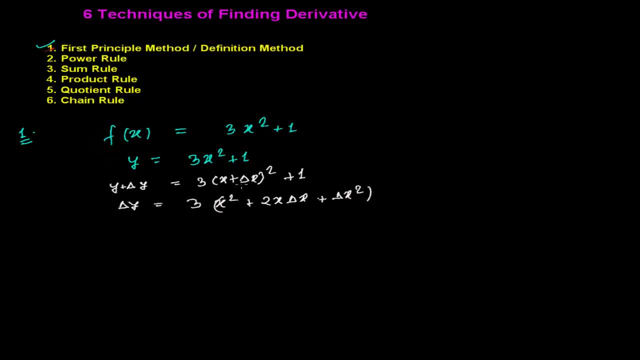 Right, I just explore this by using formula a plus b whole square, That is, a square plus two, a plus b square, And then plus one and then minus right, this y part, And then again what I can write. I can write: delta y equals to three x square plus two x, And this, this three and this two will multiple, So it will be six x times delta x, And then three times delta x, whole square plus one. And then in the place of y, I'm just saying: 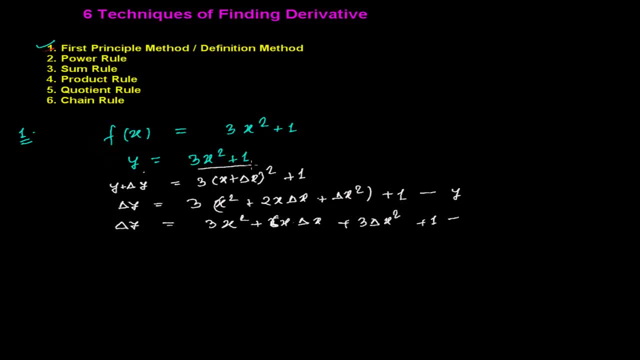 I can use this. I can use this. actually, y is 3x square plus 1, so I'm just putting here 3x square and plus 1 it is. so here is minus. that's why I'm writing here minus 1. now I'm sure there will be. 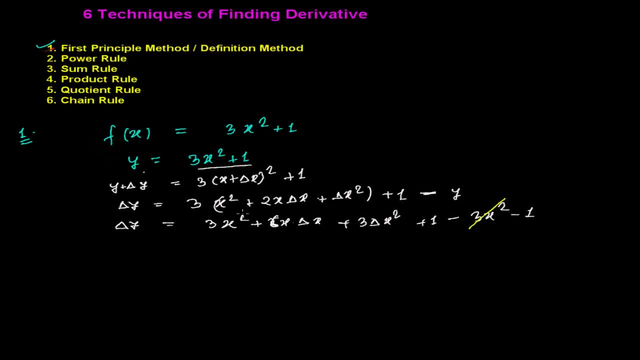 some cancelling parts. see here: minus 3x square and plus 3x square. similarly, minus 1 and plus 1 will cancel out and now we are left with few things. that is, delta y is equal with now actually 6x times delta x plus 3 times delta x, whole square. I think I can take the common from here. 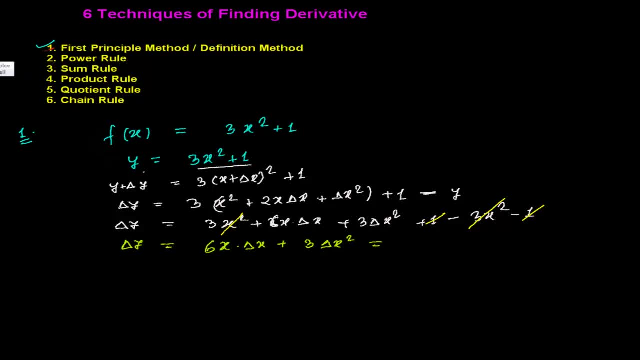 right, we used to every time. I know I think you're remembering- every time we used to take the delta x common. so delta x is getting common here. so that's why we're getting 6x plus delta x here now. you know, after this step, every time what we used to do. we used to divide both side, left and 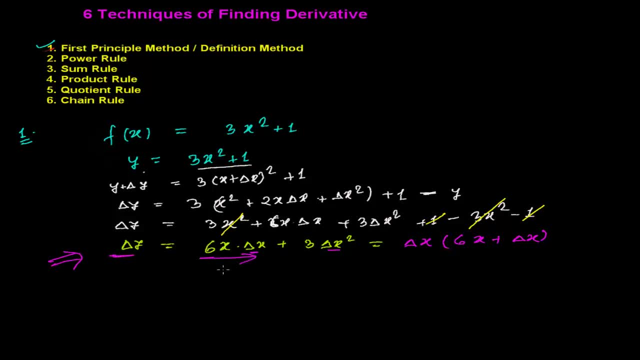 side, this left hand side as well as this right hand side, by the delta x and we have to take the limit. so I'm dividing this side also, delta y over delta x. I divide here this side by delta x and this side also I'm going to divide by the delta x. so delta x, 6x plus delta x and I divide by the delta x. this. 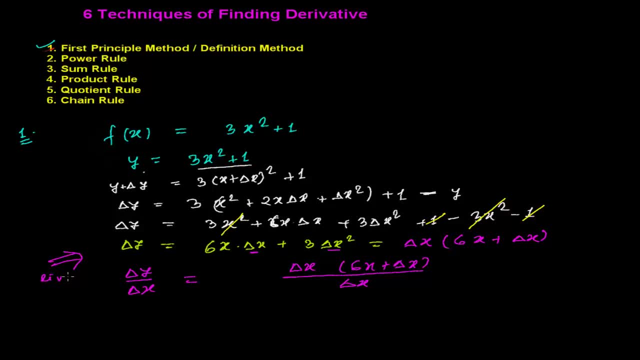 now what I'm doing. I'm going to take the limit. both side limit I'm taking right as a delta x times to 0. so this side also I'm taking limit as delta x tends to 0. so now see what I'm going to get. 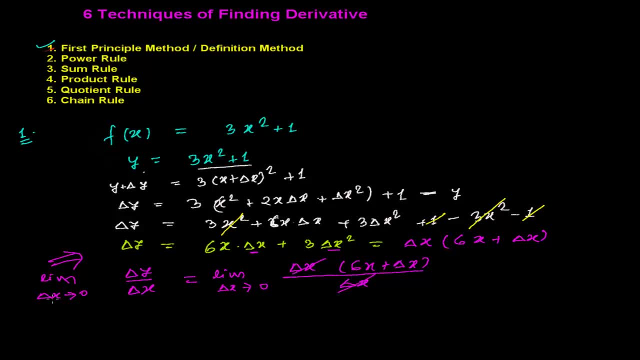 I'm going to cancel out this right and this limit. when delta x tends to 0, delta y over the delta x is actually the derivative of function y with respect to x. you can write like f prime of x equals to 6x and in the place of delta x now it will be 0, so it will be simply 6x x. so 6x times delta x plus delta y is equal to x. 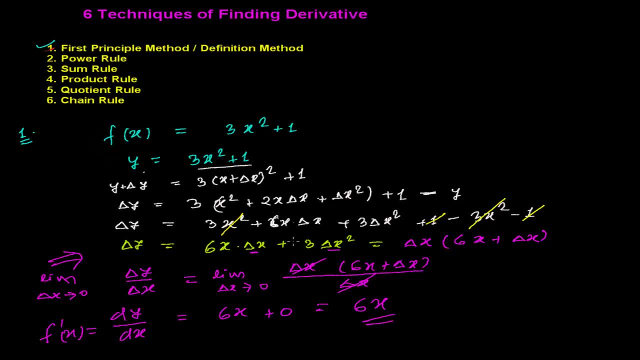 is our derivative, this, this method, like in this method, if you are finding out the derivative, this is called first principle method. but you know, uh, people start using very shortcut to find out the derivative. uh, by first principle method. also, by using the shortcut or shortest one, you can say: 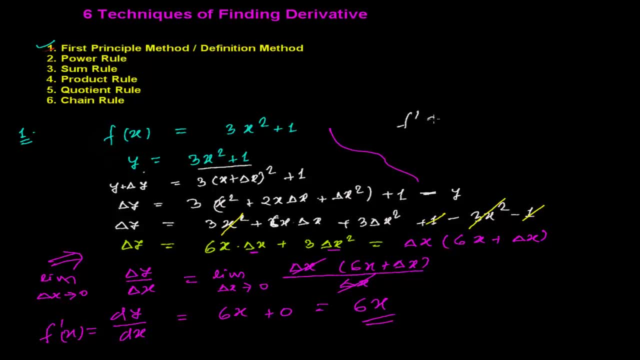 directly using the formula like derivative of a function. f of x is actually limit when delta h tends to zero. f of x plus h minus f of x, whole divided by h. this shortcut, uh uh formula you can say we might have used. yeah, we have used in many of the videos, in initial videos, to find out the 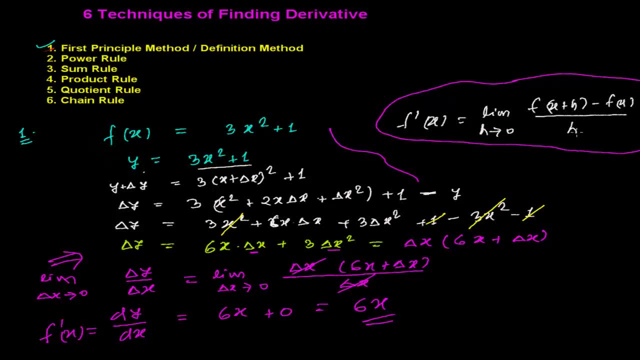 derivative. this, if you can directly plug the value here here, h is actually, you know, uh, a small change in x. or you can say in the here in this place, many, uh people, many books, history write delta x also right, so if i'm writing here x plus delta x or x plus s, that's the same thing. 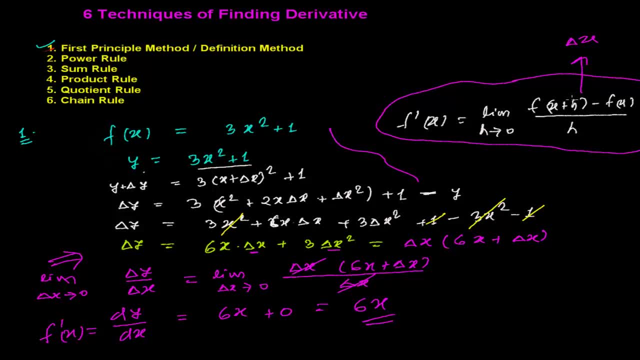 h. you just understand. there is a small change in x, a small increment, maybe decresement, whatever it is right in x, all right. so you can easily find out the derivative of this uh here also. so it will be simple like x plus h. it is so like uh. you just make a small change here, right, and you can easily. 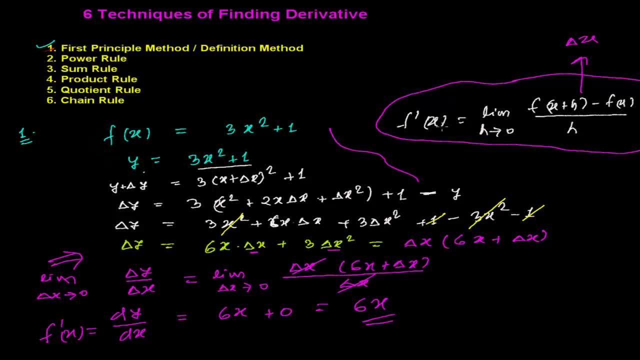 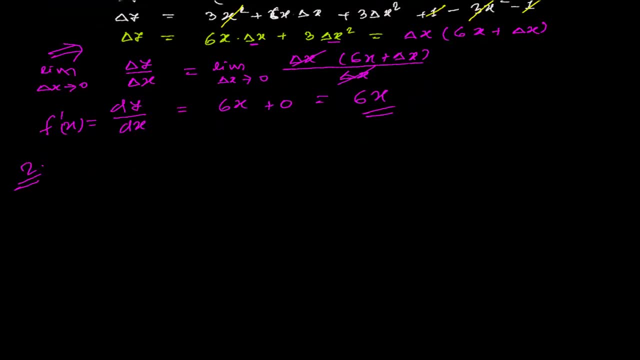 find out. that's not the way. so this was our actually first principle method, or you can say definition method. the second method was our power rule. let's talk about the second method and in power rule, what we have learned. if we have a function f of x equals to something like x in the power n, then the 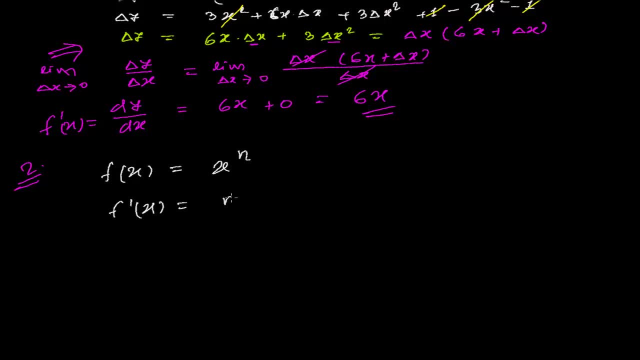 derivative of this function. f of x is actually power times x to the power, n minus 1 times. derivative of the base. whatever we had, whose power is actually n divided by dx and finally what we're going to get. both are same, so we were getting n times x to the power. 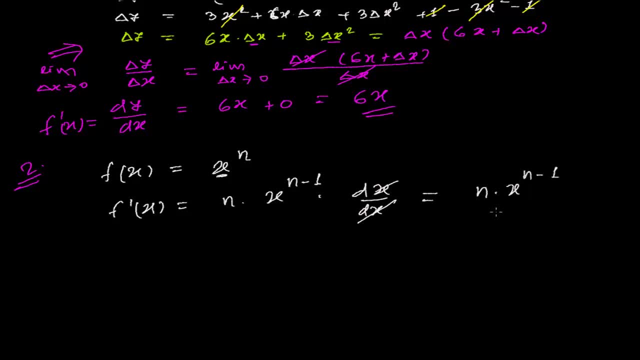 n minus 1, and this was actually power rule. and if you're finding out the derivative by using this rule, then uh, that we can say that the derivative finding by the power rule. so simple. i'm giving a good example here. suppose i have a function. uh, y equals to f of x. also, you can write. you can write. 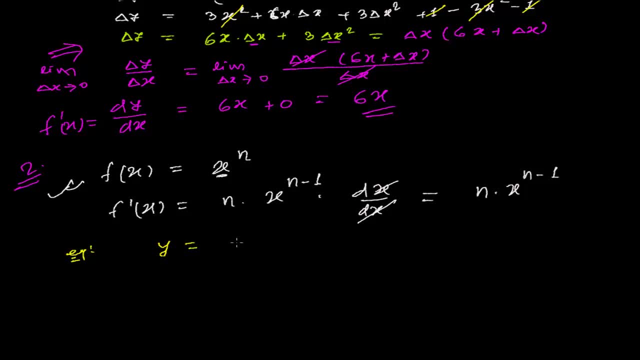 y equals to also right that same thing. um, let me say this is 3x squared plus 2 whole to the power 4, right? so in this case, what i have to find out, derivative, right? so dy by dx. or you can say derivative of the y which is reduced. x is now c powerful, as i said. 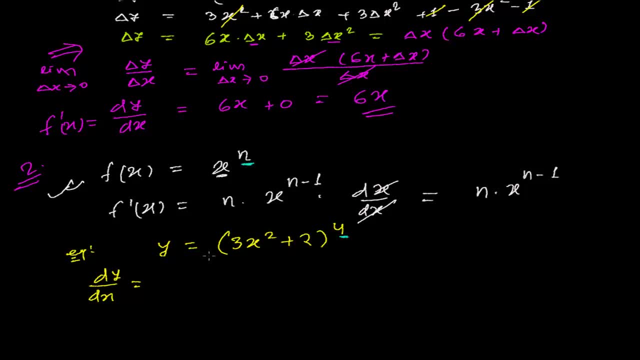 what is my power here? power is n and here is 4. so first i'm writing 4 and then, whatever the base i do have, that is x, and in the place of x we have here now 3x square plus 2, so 3x squared plus 2. 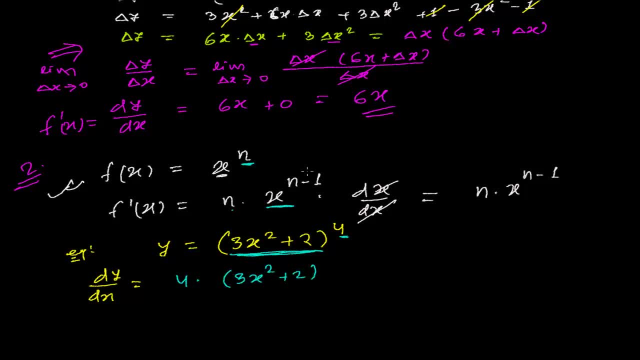 square plus 2 whole to the power whatever. in the power there will be one less, right. so 4 minus 1 less. and then times derivative of the base, whatever we have with respect to x, right, so our base is 3x square plus 2 whole divided by delta x. and finally we're going to 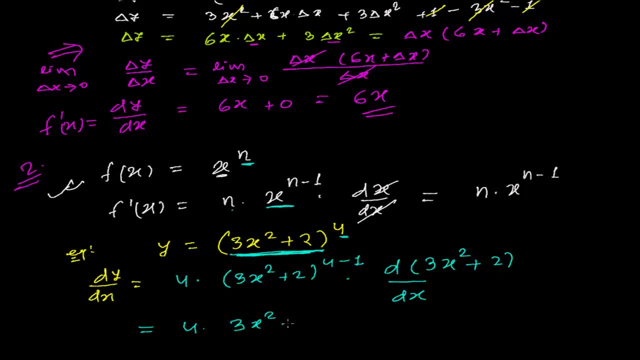 get like 4 times 3x, square plus 2 whole divided by- sorry, whole to the power, 3 times now, derivative of this function will be what? 3 to the 6 right, 2 minus 1, that will be 1. so I don't have right. 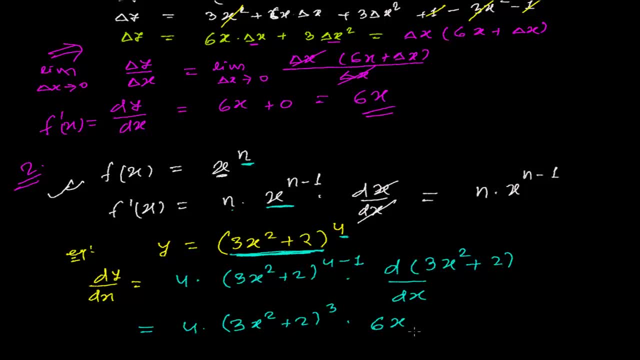 like derivative of 3x square plus 2. you have already found out that is 6x. so that's why I'm writing here directly: 6x. all right, here also, actually I have used the power, uh power rule here also, simply in a short way I have used. let me show you I've just how I had find out. 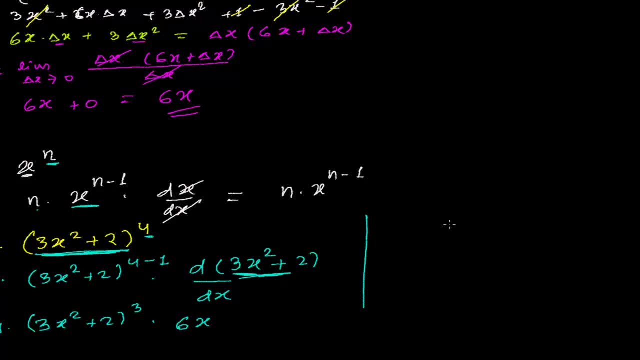 what I have done here. so I have used the power, uh, power rule here also. simply in a short way, I the derivative by using power rule here. like our function is here, y equals to 3x square plus 2 right, and therefore dy by dx. I'm going to say derivative is, this is the constant, so I need to. 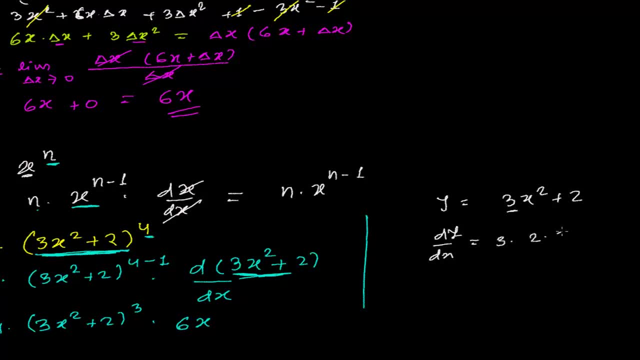 put outside right and what is the power is here 2, so power times, whatever the base, and we need to raise the power. less 1 right, 1 less we need to raise. so initially power we had 2 here, so there will be now 1 less. 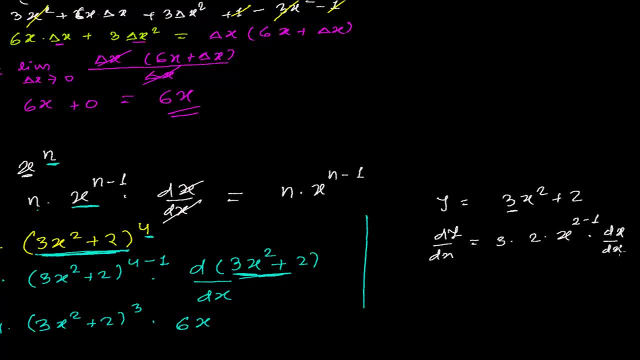 times, dx by dx, but generally people don't write this and actually they're gonna cancel out. so that's why, directly you can write 6x also, but you need to first. you need to do a lot of practice, lot of practice. once you get perfection so you can directly write, you know you don't have to do these. 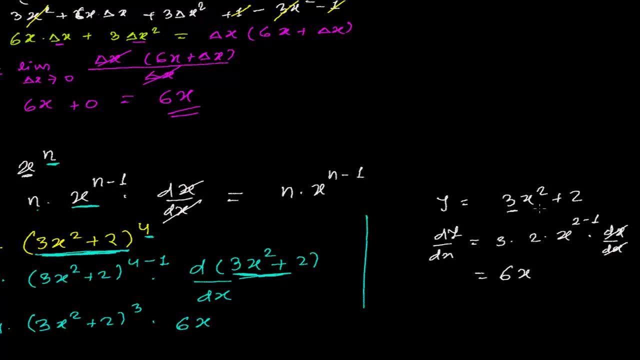 all steps directly like: find out a little bit: derivative of y equals to 3x square plus 2, then that time you can easily do like: dy by dx equals to 6x. but for that, you know, you need to do a lot of practice, a lot of practice, and I hope you're doing good. 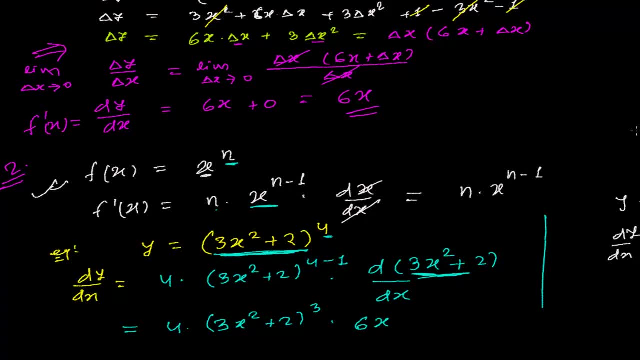 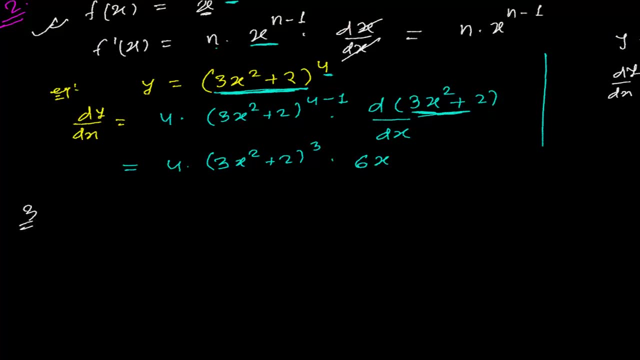 all right, so this was all power rule, and the next rule is sum rule. all right, so the third one, let's talk about sum rule. in sum rule, you know, suppose I have a function h of x equals to f of x, plus another function g of x. if two functions are going to be added or subtracted, that doesn't. 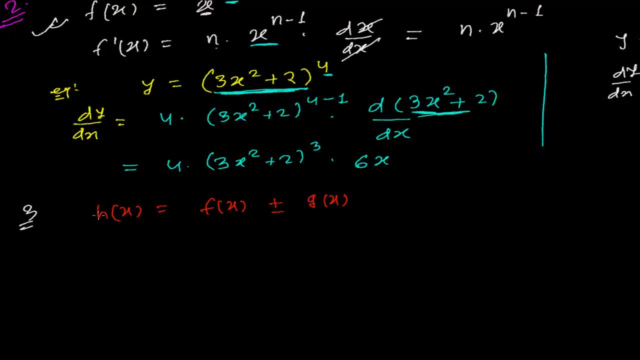 affect. so how to find out the derivative of this? now, h of x, these functions. so for this, nothing is there. simply, you know, derivative of the h of x is actually derivative of the first function plus derivative of the second function, right? so first find out derivative of the first function and 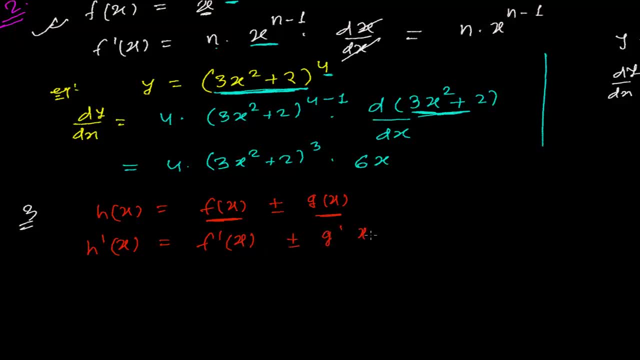 then plus, minus, derivative of the second function. you know already that, like writing here, prime means derivative is that. and for that I just want to give a very quick, simple example. well, suppose, and gx, you can say let me give x to the power 5. well, well, I need to write this x to the power 5 first. 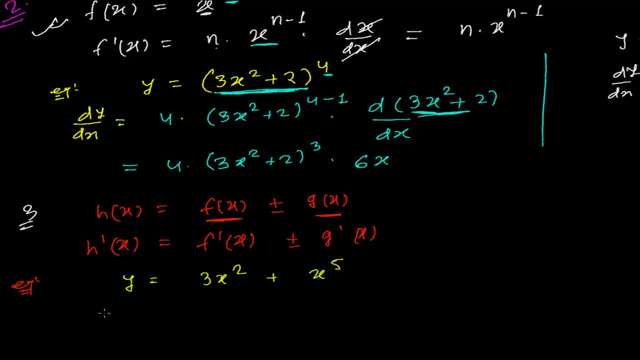 and 3x square later. well, no problem. so now, derivative of this function. y. simply, you can say like dy by dx is. now I'm again using the power rule, the same method. I just want to tell you what is the method right? so first I need to find out the derivative of this thing, right? this is a. 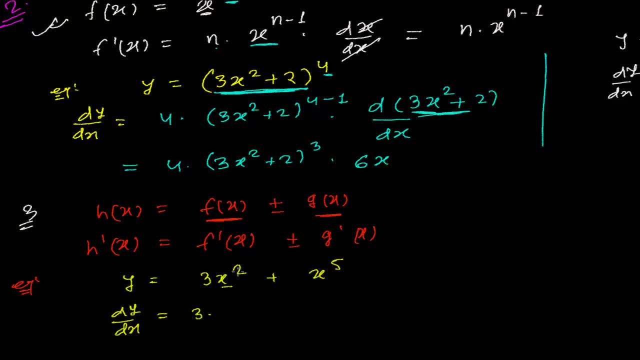 constant, it will come outside. so x to the power, 2- I'm using the power rule, power times base and 1 less in power. and dx by dx, like here, will be derivative of a rule x to the dx by dx. so i don't think i need to write it all right, but it is initial state, so that's why i'm writing well. 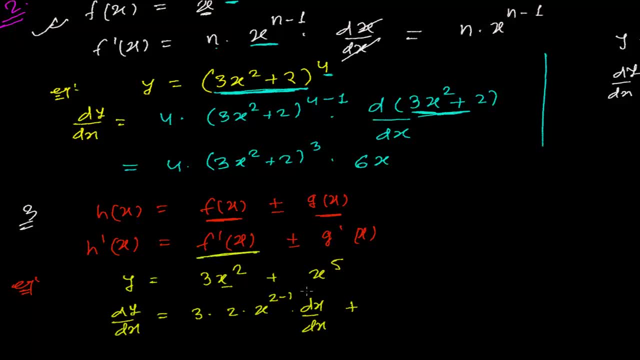 now again i find out the derivative of this. actually, if f of x, i already find out here, now i'm going to just find out the derivative of x to the power 5. so again i'm using power rule, that is, power times, whatever the base i do have. just i need to make in power 1 less, so 5 minus 1. 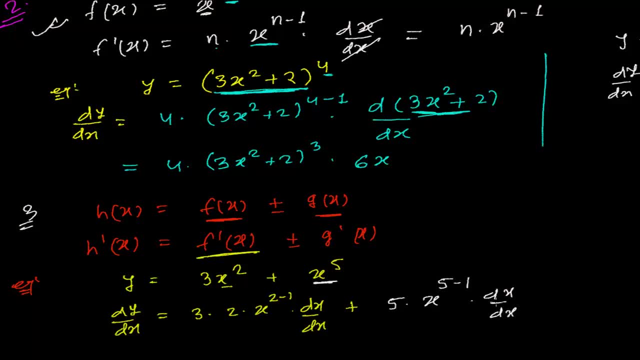 times again: dx by dx. we don't have to write these things. actually you can cancel. if you don't want to write, don't write. nobody will say you anything, because everybody know dx by dx is 1, right? so 3 times 2, that is 6, x and 2 minus 1. we don't have to write now 5 and x to the power 4, right? so this. 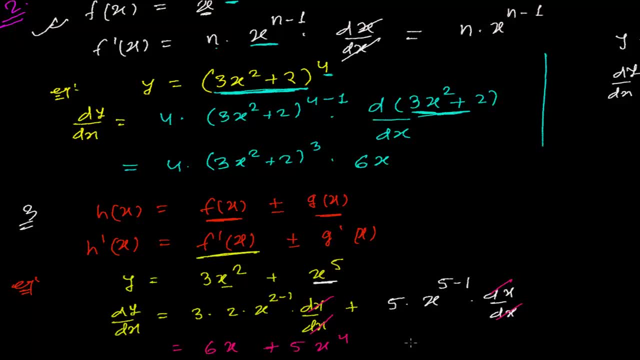 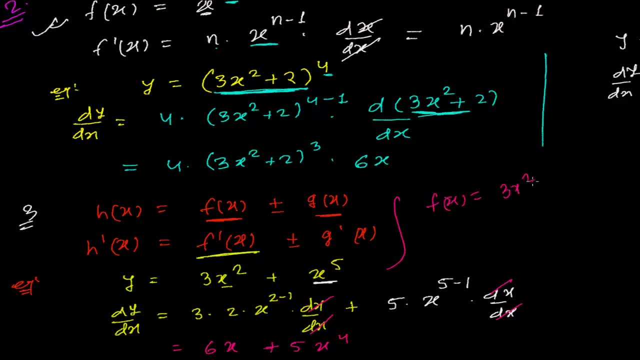 f of X is a function which is 3x, square, and G of X is another function, which is actually X to the power 5, right? so in that case, these two functions are going to be added here. they're here, maybe minus or plus, that doesn't affect I. 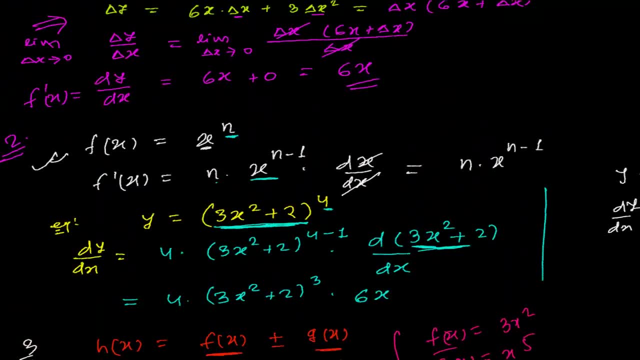 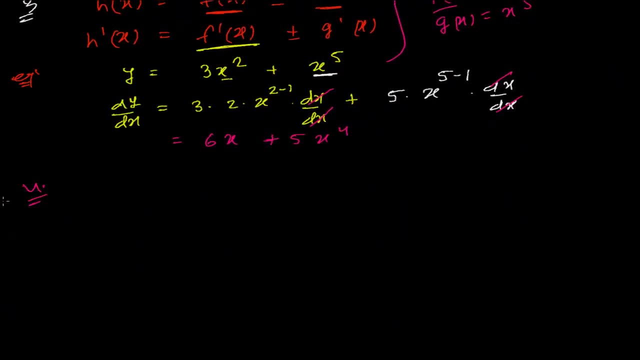 already told you, right? so this was our sum rule and now we are going to learn about, I think, product rule. well, this is a little bit important, so let's talk here: product rule. so what is product rule? you know very well. like I have a function, like y equals to suppose function f of X and G of X, I don't want. 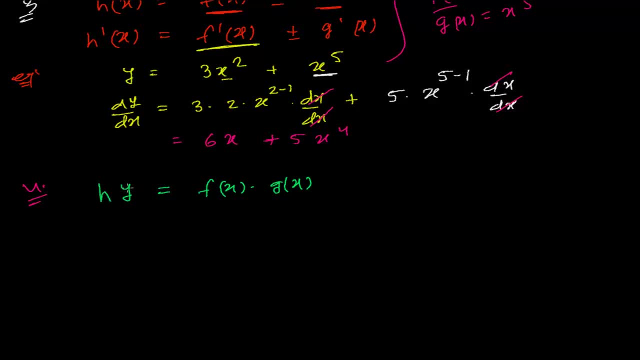 to write this at a Y. let me say this is H of X. right, this is X. H of X is another function which is the product of actually two function: f of X and G of X. so, in that case, how you will find out the derivative of this? well, let. 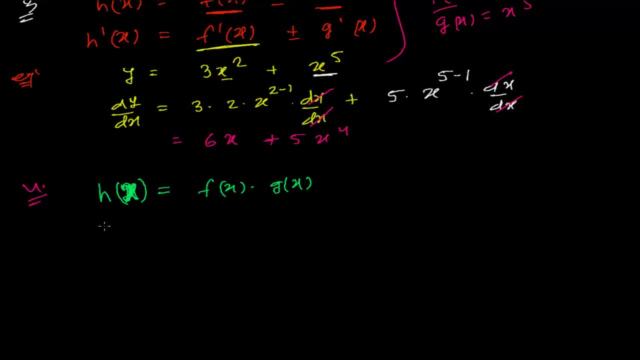 me take an example. and now, first let me write the formula, what we used to do. actually, the derivative of the function H of X will be first function times. derivative of the second function, again derivative of the first function times, second function. right, many people write like this also, like you know, if you have. 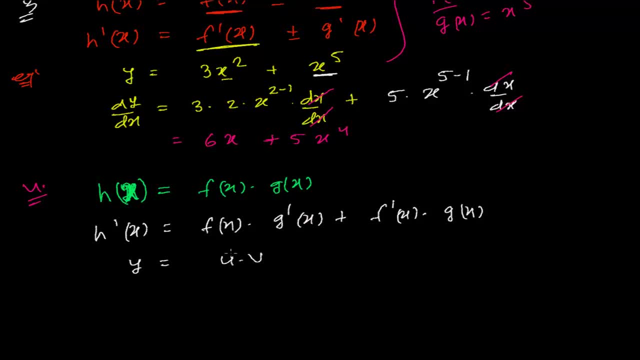 something like y equals to U and V represent. here U and V are representing one individual functions, so that time derivative of this function will be first function times derivative of the second function with respect to x right, and again second function times derivative of the first function with respect to x right, when 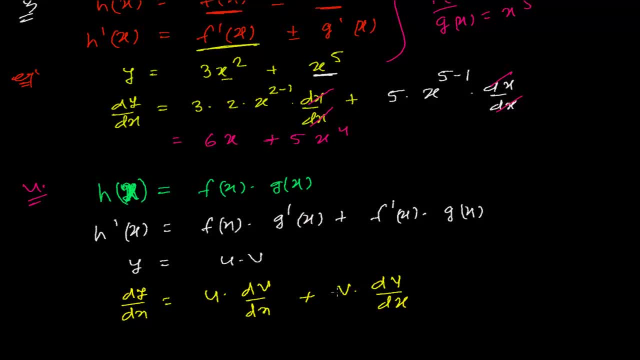 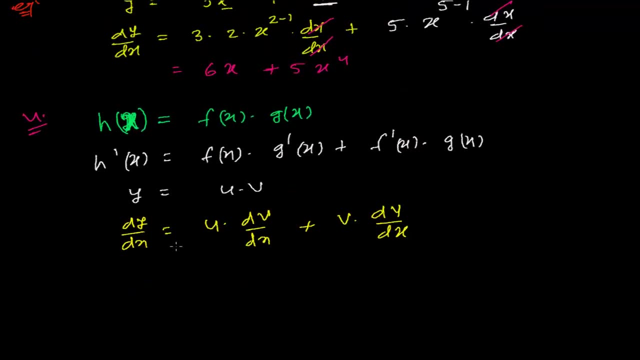 you're taking first function, there would be- will be, second function when you're taking second function. there you really have the first function right. so that's not the problem. it's very easy to quickly remind you know. uh, you can say like derivative of the function y to 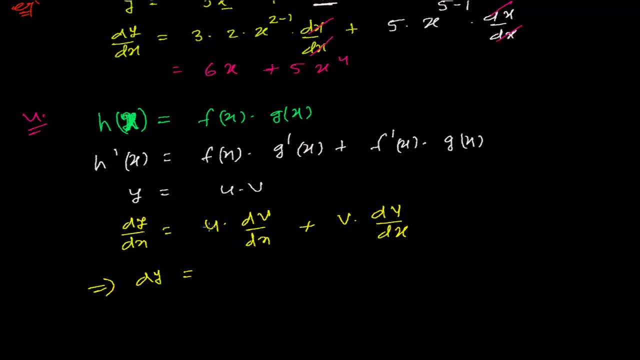 quickly remind this. another formula: well, uh, to, just to remind u, dv, right, you can imagine, like like u, dv and v du. all right, u dv, video, u, dv and video. u, here representing one function, and dv means derivative of the function, v, and here is v. right, this is v. well, it's very dirty. this is v and this. 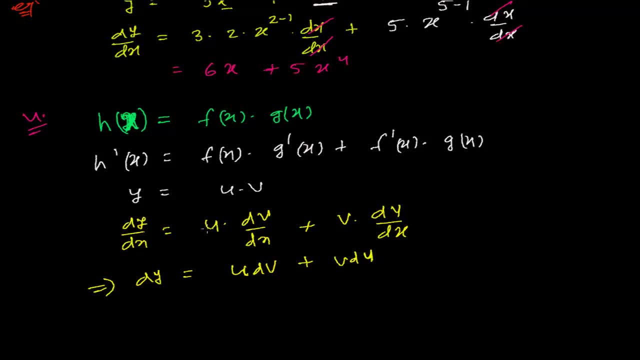 is derivative of u and even short. if you want to understand, then you can say: u audio minus video, right v du video, a u dv audio. something like you can say: audio plus video, right audio plus video, like something like this. i used to remember something like this. well, uh, you can remember. 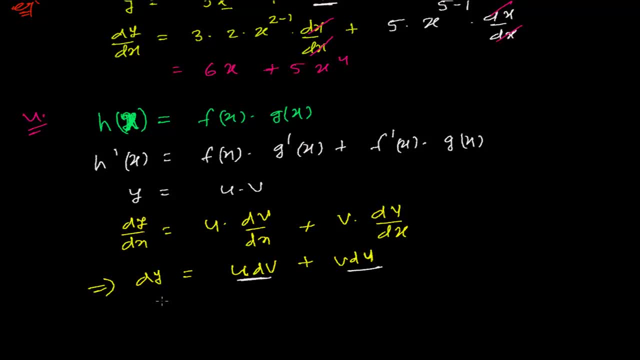 in any ways. simple it is, but let me give you a simple example here, right? so So suppose example. let me give you here. suppose I have a function: y equals to 3x square times. right, this u is one function which is 3x square. or you can say: fx is one function which is 3x square and another function. let me take x plus 1, right, x plus 1, this is another function. this gx is actually x plus 1.. 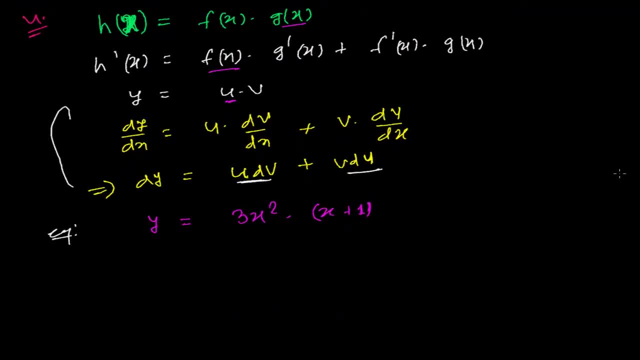 So two function is going to multiply here. So now how to find the derivative of this? So to find out the derivative of this, simply dy by dx. as I said, write first function right first. write first function, then find the derivative of the second function. So I'm writing first function and I'm going to find out derivative of the second function, x plus 1 right. and then again write second function, find the derivative of the first function. So I'm writing second function and going to find out the derivative of first function. 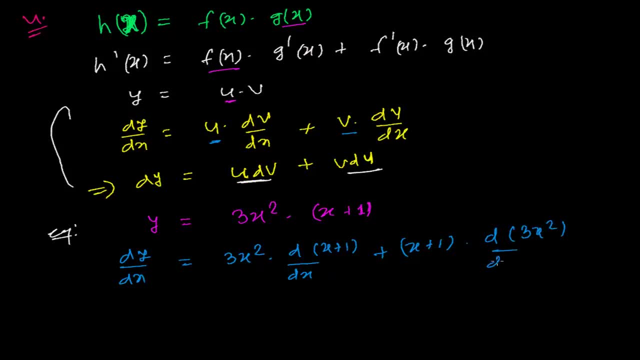 So dy by d, 3x square over dx. So now fx square is 3x square and see x, derivative of x. now you can use here some rule. first, derivative of x, dx by dx, that is 1, and derivative of a constant, that is 1 is a constant. derivative of constant is actually 0, right and again x plus 1 and here 3 is actually a coefficient, so it will come outside and x square. 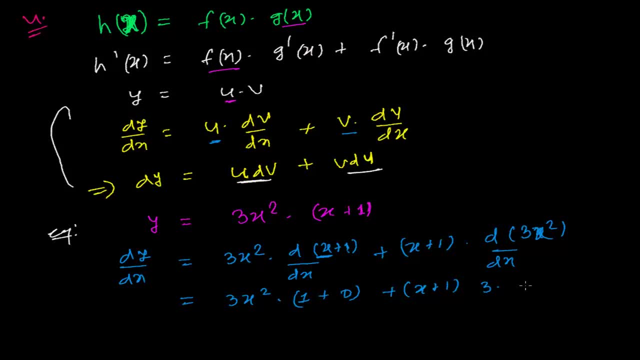 So it is right x square. so derivative of x square is 2 times x to the power, 2 minus 1, right 2 minus 1.. So finally what I'm getting? I'm getting 3x square plus 3 to the 6x and in the bracket x plus 1 you can open it also: 3x square plus 6x square plus 6x. Finally I'm going to get like 6 plus 3, 9x square plus 6x. This is my derivative. 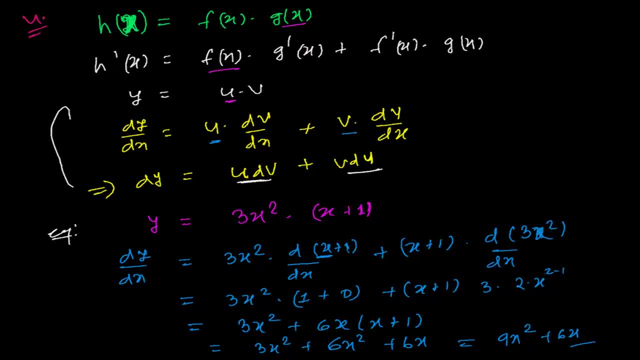 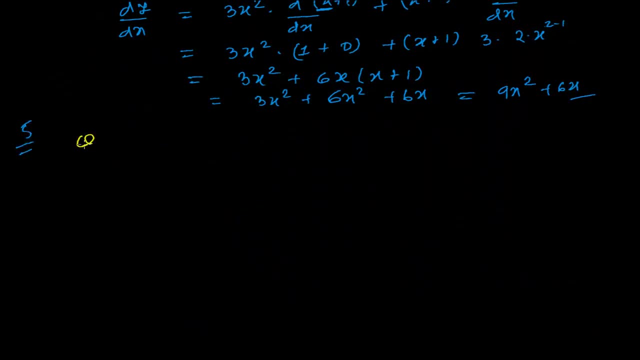 Right, using, using using product rule, and after that we had learned another rule, that is it's, I think, fifth quotient rule, right? So what is quotient rule? Well, quotient like something like two function we have in the like dividing form. like I have a function, f of x, which is going to be divided by g of x, another function, and now it is another function, h of x. 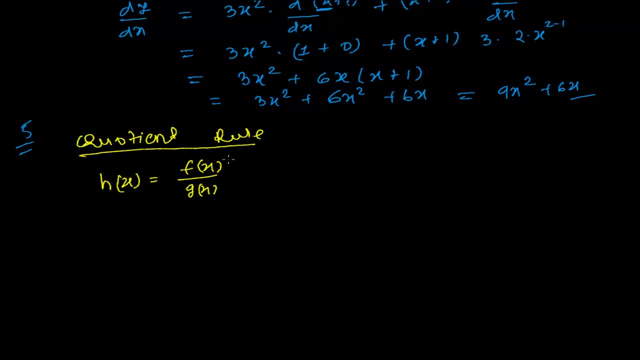 So h of x is going to be divided by g of x. So h of x is I have a function which is actually the one function divided by another function, right? So in such cases, how to find out the derivative of this function? So we had learned the rule. actually, I'm revising these all things I know you might be knowing, just I'm reviewing, all right. 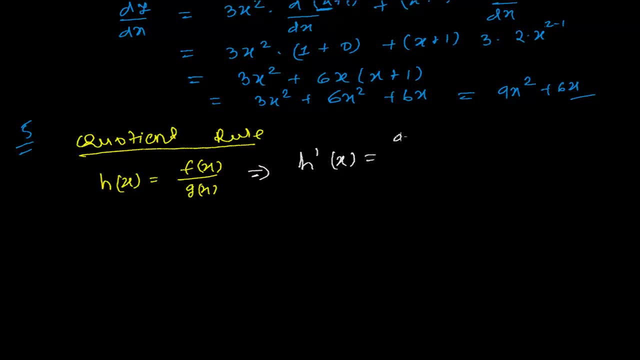 So it is simple: second function, right? second function times. oh well, how bad it is looking. second function times- I'm talking about. this is my second function. Second function times: I'm talking about. this is my second function function. this is my first function. okay, so second function times, derivative of the first function. 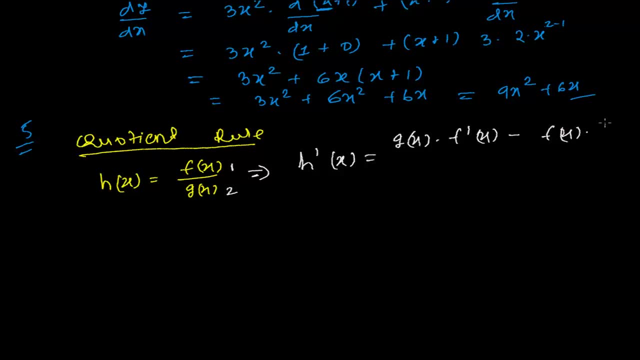 minus first function, times derivative of second function, and then whole divided by square of the second function, square of the second function, or in the form of u and v, if you want to see. i feel easier there. i don't know why. well, i have a function, u and v, suppose. so what will be my 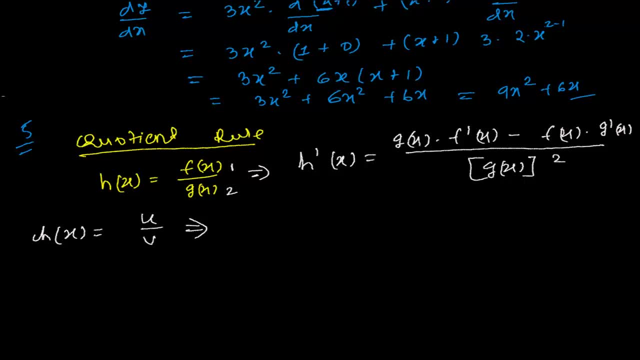 derivative now. so my derivative is going to be v times derivative of the uh u and again sorry, here will be minus right u times. derivative of v means second function divided by v square. okay, so v d? u minus u dv. divided by v square, so vdu. now you can say video minus udv audio. 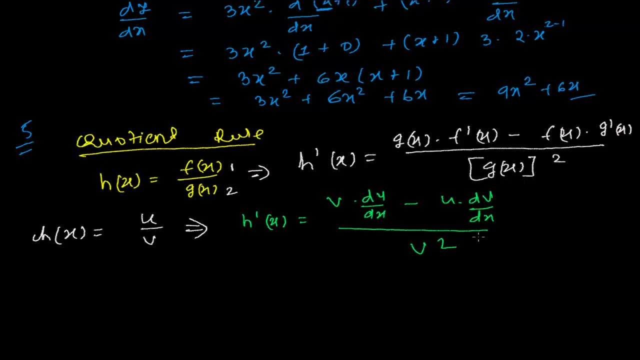 over v square video minus audio. over v square video square, something like that. all right. well, this is just a trick. however you wanna remember, it may be crap, someone, maybe some people you may not like, right well, this was my uh way of learning. leave it well, so simply vdu, uh du over dx and u. 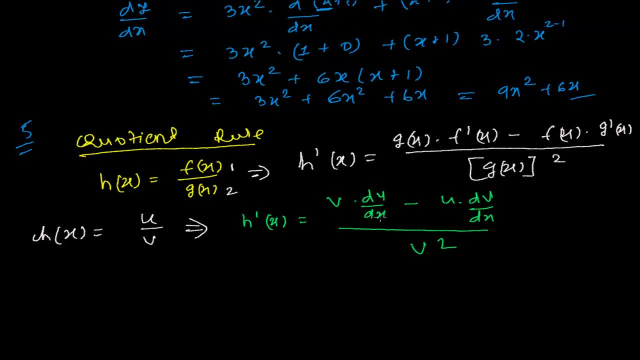 dv over dx, because i'm going to differentiate with uh, with uh with respect to x, right? that's why this is the formula. so i'm going to give a very simple example here. very simple, right? uh, what should i give? well, suppose i have a function. y equals to. 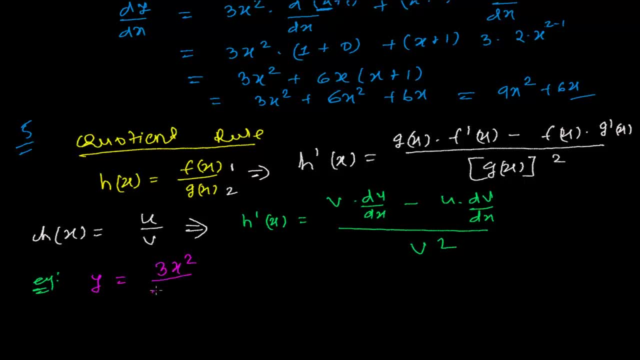 uh, 3x square over um 2x plus 1, right. so here 3x squared is representing function u, or you can say fx, and 2x plus 1 is representing function gx, or you can say v. all right, so now we have to find out. 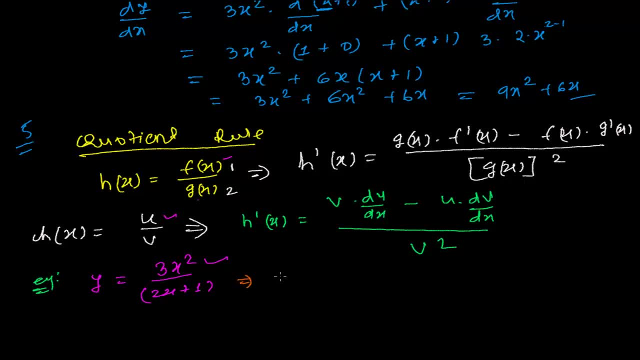 the derivative of this. so therefore, what i'll write now, that derivative of the function y, with respect, equals to, again, second function as it is written here, right, second function: 2x plus 1 times derivative of the first function, D, by TX of 3x square. all right, 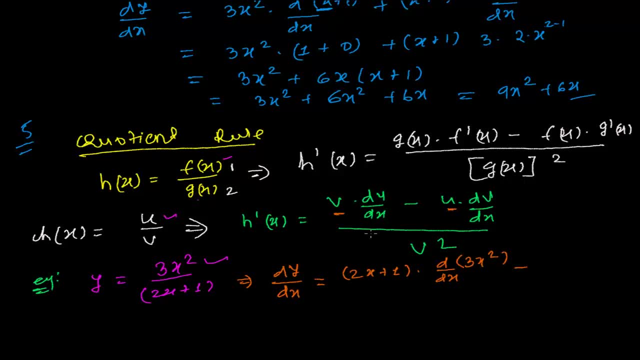 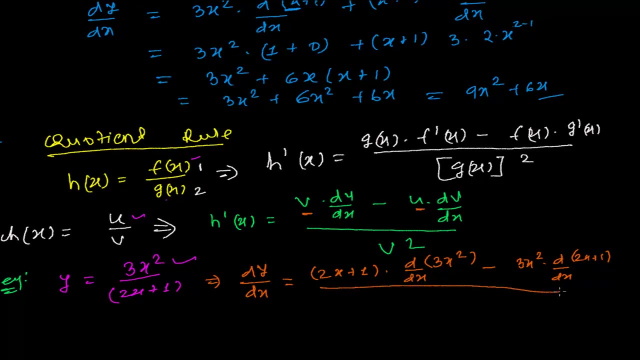 and then minus CAU. that is first function right, 3x square times derivative of the second function, that is 2x plus 1. well, let me shift a little bit. well now, whole, divided by now square, of the second function. but you can see the. 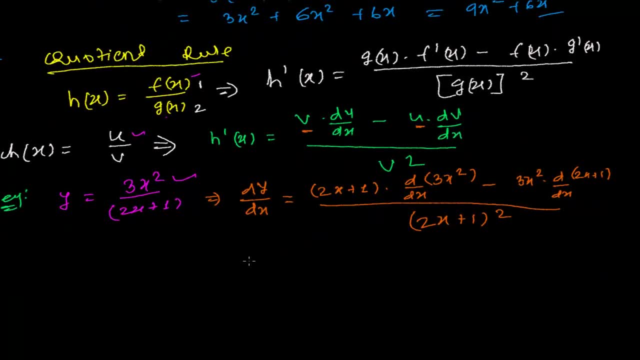 square of the denominator. all right, so now what I will get. I will get my derivative as now: 2x plus 1. it is right, 2x plus 1 times now derivative of 3x square is actually X. now your export, I know that. and 3 X square, it is 3 X square and derivative. 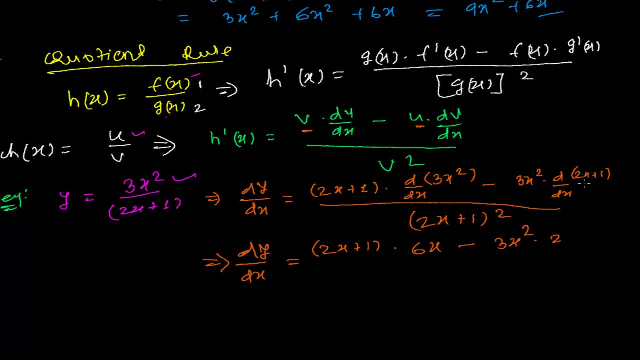 of 2, X is just like C coefficient and derivative of X will be 1 and derivative 1 will be 0, so I'm not writing those things. alright, and whole divided by 2, X plus 1, whole square. and now you can like, you can multiply and you can solve this. 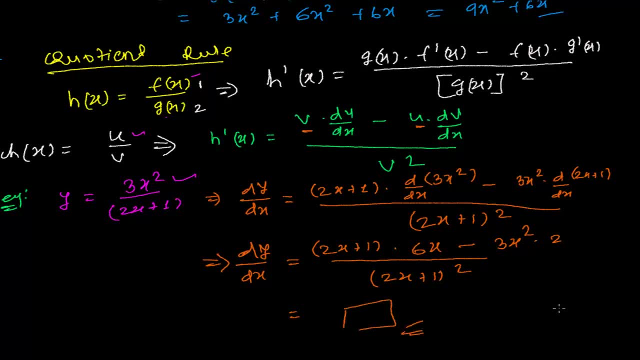 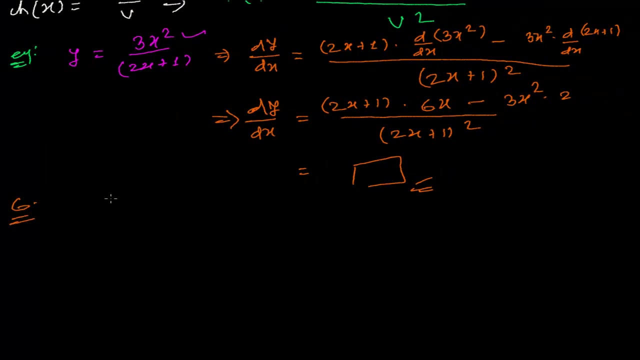 expression and finally you'll get derivative. alright. so I was just talking about the rule or technique, what we had used and further, what we are going to use now. the last one I just want to tell you here that is called chain rule. right, the sixth one, and it is also very important rule that really plays a very 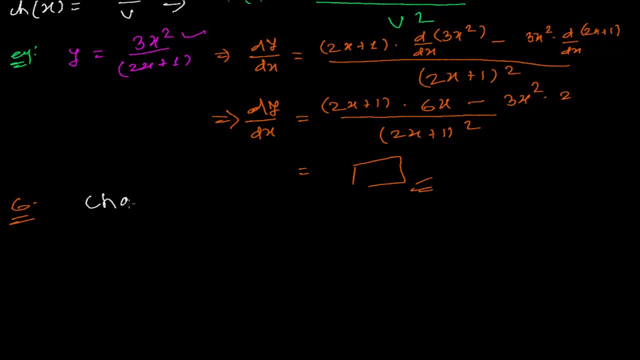 important part while solving derivative. it's called chain rule. so what is chain rule? so chain rule is, you know, a little bit different than other, as we have learned, because in here, in one function, other function get attached, you know, get enclosed. suppose you have a function that is closed and you have a function that is. 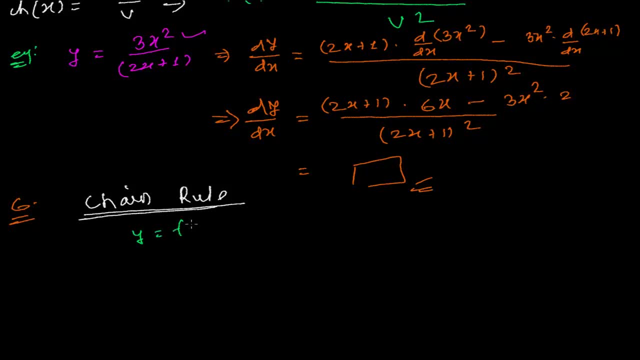 closed. I have a function something like Y equals to F of you see here, where you know where actually you is also another function, something like GFX, so in that time, how to find out the derivative you know. so actually we had learn like it is something. if if we have such condition, then dy by dx will be actually. 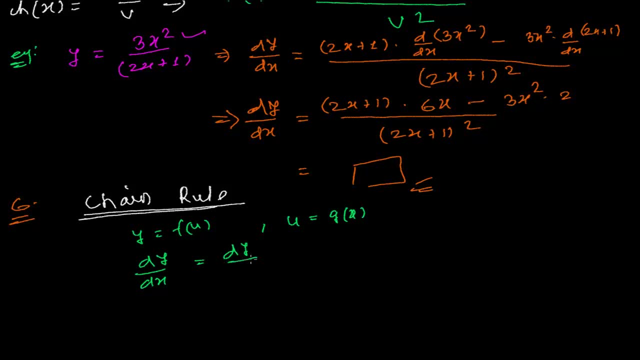 derivative, the function derivative of Y with respect to you, right, derivative of Y. derivative of function Y with respect to the derivative of Y with respect to you, with respect to you, times. derivative of function u with respect to x, with respect to this X. try to catch it so in this way, actually, ways to find out, and 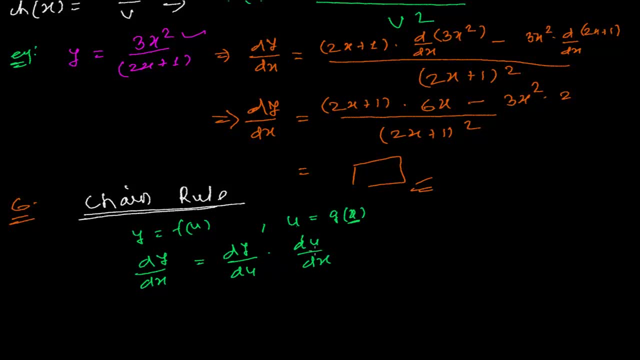 finally, you know what happens actually. you going to cancel a lot of things here and you will get the result finally. and you can simply also say like this is dy by do. or you can say like: do by or DX, you know, dy by, do you? if you say like: 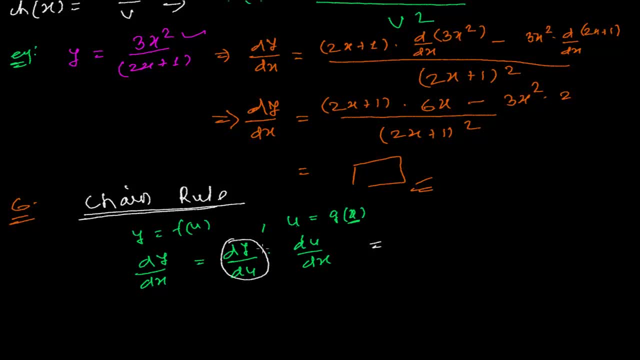 sex with this function. you know this. if you, if you in the place of this, you can write also like something like they: video of the first function times du by dx. you know it will be a little bit un-understandable. let me take a good example. suppose i have a function. well, let me let me think. suppose y equals to 4 u square. 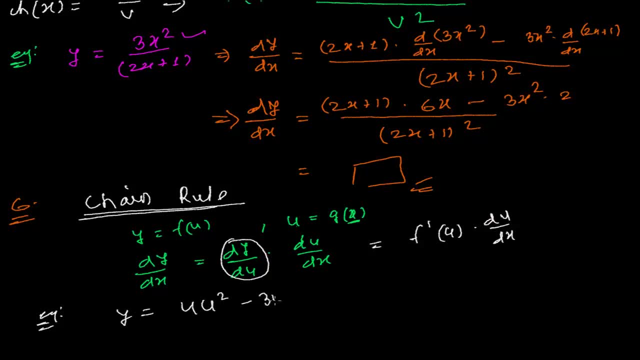 this is right: 4 u square minus 3 u plus 5. suppose this is my function and i i told you like here: y equals to 4 u square minus 3 u plus 5, and u is itself another function, right? so let me suppose. 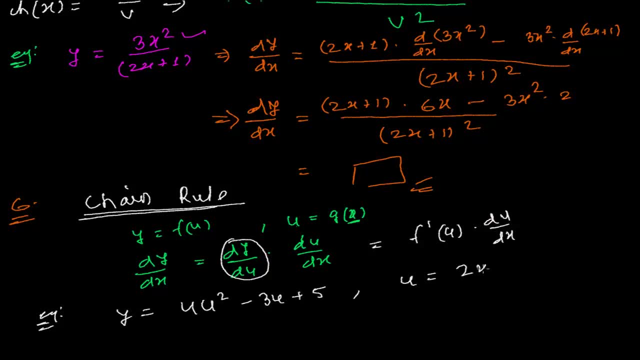 here u is actually. you can take anything like 2x square minus 3. now how to find out the derivative of this? so i already told you, in this condition, to find out the derivative, we have to say: dy by dx is actually. now let's see here i'm just going to write dy by dx first. dy by dx, sorry, dy by. 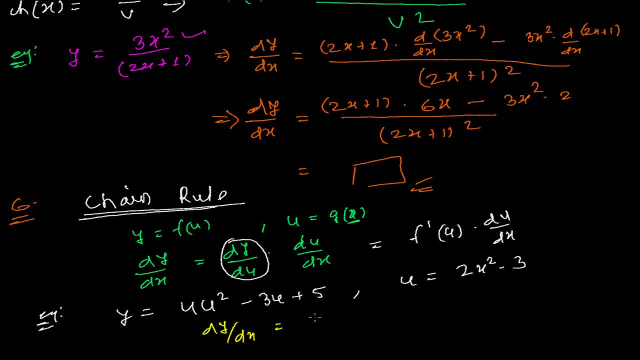 d y by d x. i'm just first going to write derivative of y, this function, right. or you can say: this function with respect to u- see with respect to u. times again, derivative of u. now, derivative of u with respect to this x. with respect to this x. right, same thing how i'm doing. let's check it out. 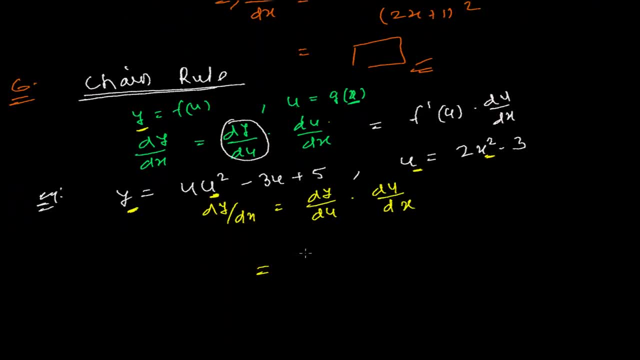 uh, now dy by dx, so derivative of y. that is what. 4 y by dx. there is nothing. you can write like 6, four times y, therefore derivative of u with respect to u, this times derivative of y. you can write the derivative of y, this means derivative of u. 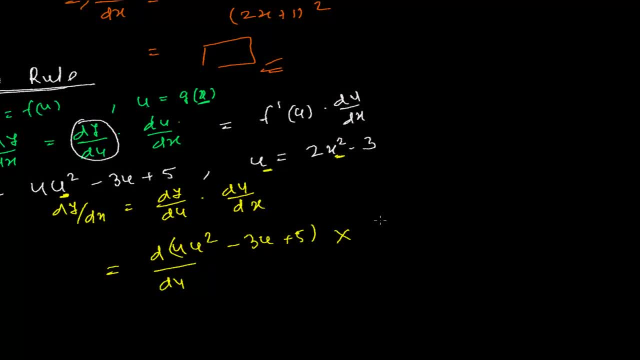 actually derivative of y, also divided by the derivative of 2 x square minus. for chapter 4. speak right sun, democratic in the axiom of predictability. right here we're going to take derivative of x, dance to x, expansion x with respect to x, add up 4 times y, so derivative 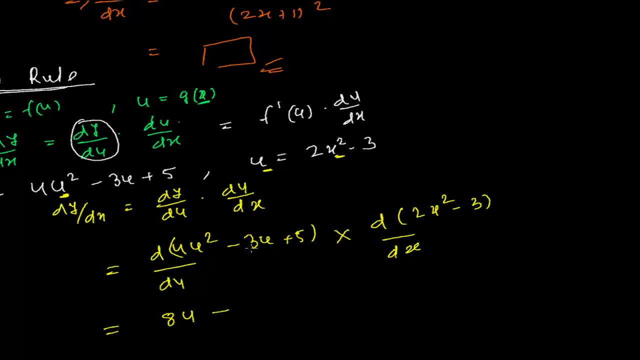 u minus derivative of 3u, it will be, since 3 is a coefficient, so it will be 3u. and again you'll get du over du, right? so i'm not going to write. well, if you want, then you can write also. and derivative of f is of derivative of this. 5 is actually 0, because 5 is a constant right. 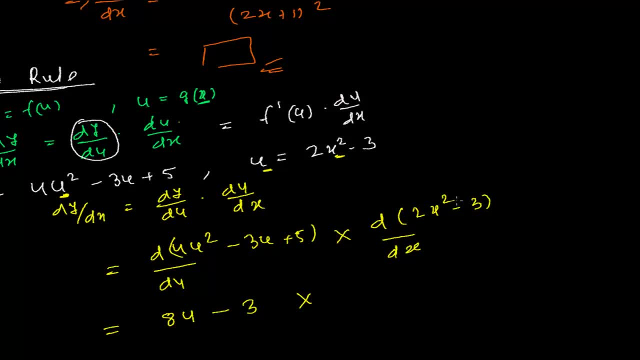 times. now see what you're going to get: 2x square minus 3. so 2 times 2, actually power rule i'm going to apply, since this is 2, right? so 2 times 2 it will be 4u, 2 minus 1 and this: 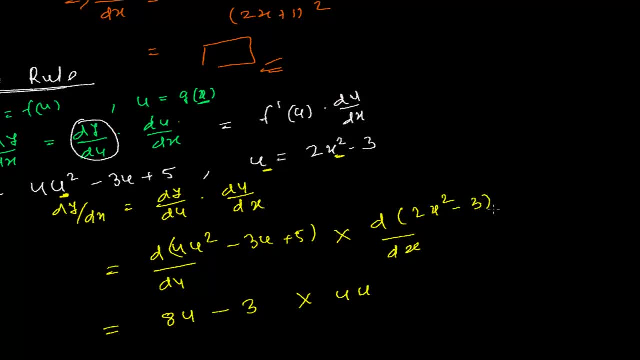 derivative of 3 is actually it's a- you can say a- constant, so that will be 0. so i am not going to write now here. now what do you get? finally? 8u times 4u. so finally, i'm just going to multiply this. 4u will multiply this whole part, right? so 8u times 4u, it will be 32u square minus again. 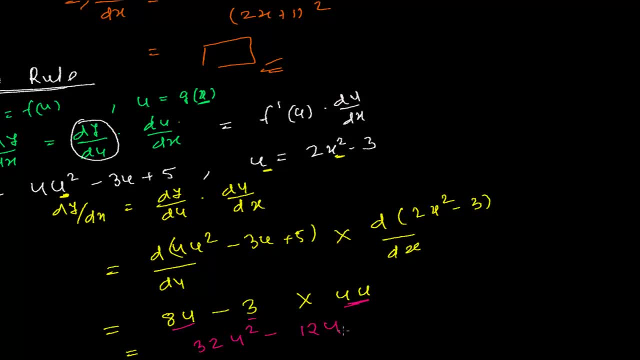 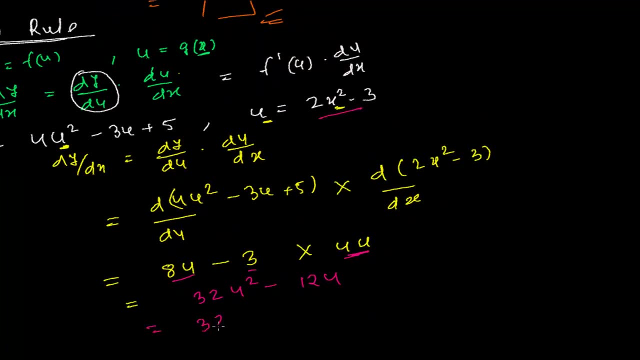 this: 4u will multiply this 3, so you'll get. you'll get 12u and let's put the value of u. that's it and the value of u have got here 2x square minus 3, so it is 32, right? 2x square minus 3, right? you finish this part and then plus.